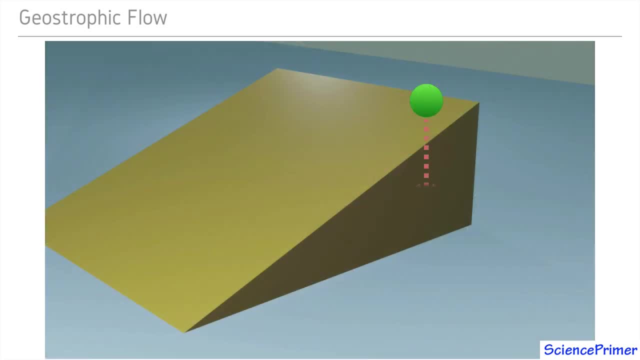 Consider a ball sitting at the top of an inclined plane. The force of gravity pulling down on the ball will cause it to roll down the plane. In this situation, the force of gravity is strong and the motion of the ball is fast relative to other forces acting on the ball. 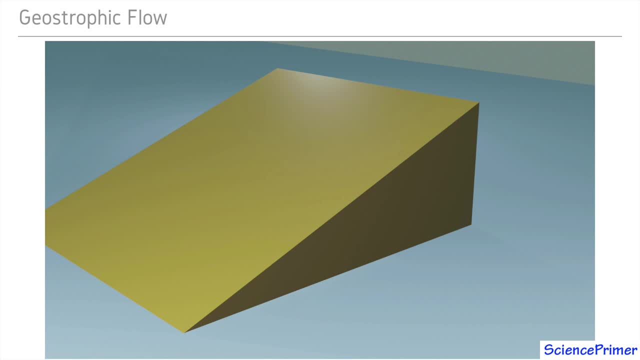 allowing the force of gravity to roll down the plane. The dynamics change if we alter the situation so that the slope of the plane is very shallow and the ball is tiny, As the slope of the plane and the mass of the ball decrease. 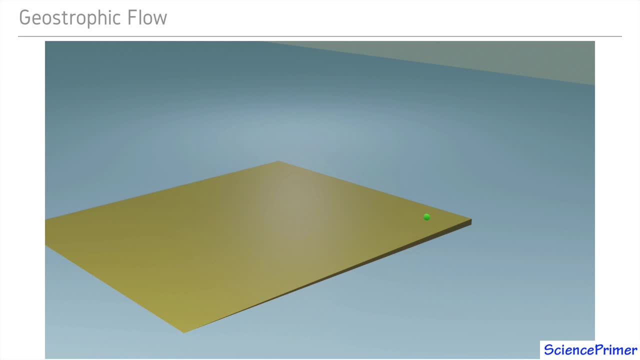 the force of gravity acting on the ball becomes weaker. With a small enough ball and a shallow enough plane, Coriolis deflection becomes so influential that it overwhelms the orientation of gravity's. pull down the slope and the ball will actually move across the plane. 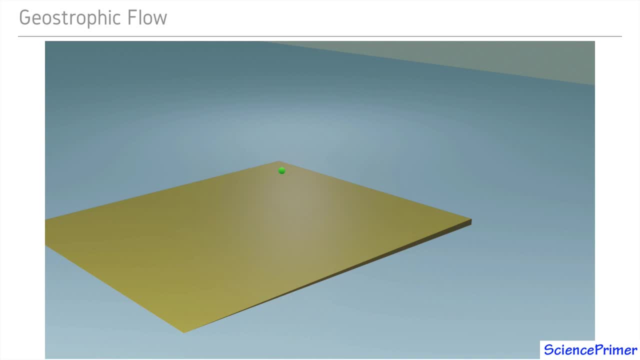 instead of down it. This can create some seeming changes in the direction of the plane, and the motion of the ball will be extremely counterintuitive behavior. If, instead of a plane, the ball was on a small hill, it would roll around the hill instead of down it. This is geostrophic movement. 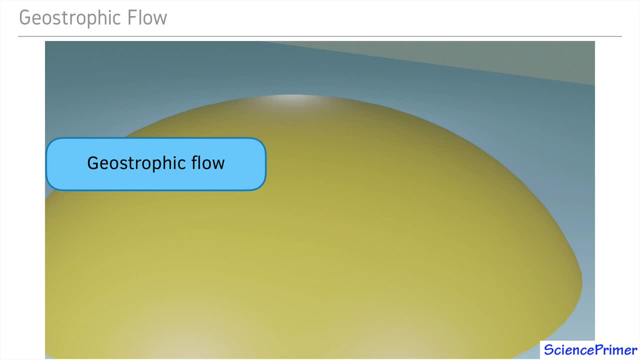 or, as used in fluid dynamics, geostrophic flow. It is important to understand that for this type of motion to occur, the slope has to be extremely small and be extended over a very large area like, for example, a large portion of an ocean basin. 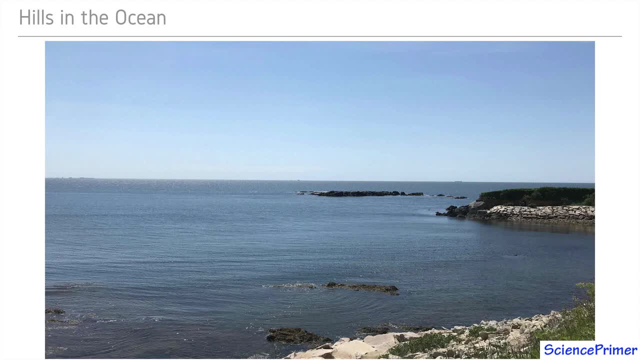 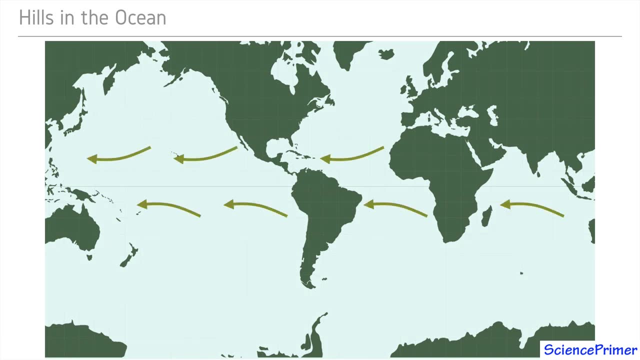 While the ocean surface does look flat to the unaided eye, there are hills of water in the open ocean. The hills form at mid-latitudes in both hemispheres, where the low-latitude easterly trade winds are replaced by westerlies at higher latitudes. 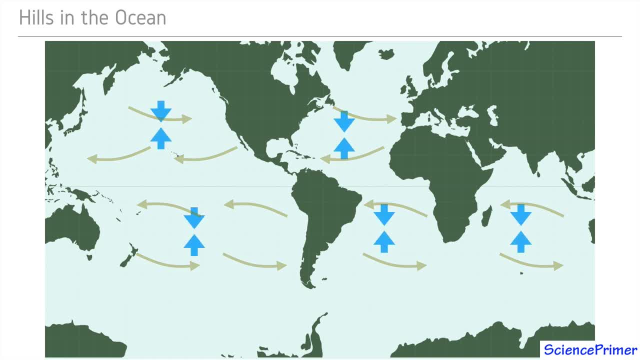 The surface currents created by these winds are turned 90 degrees by Coriolis deflection. The resulting Ekman transport drives the formation of regions of convergence where water actually piles up, forming small hills. These hills of water are only about a meter in height. 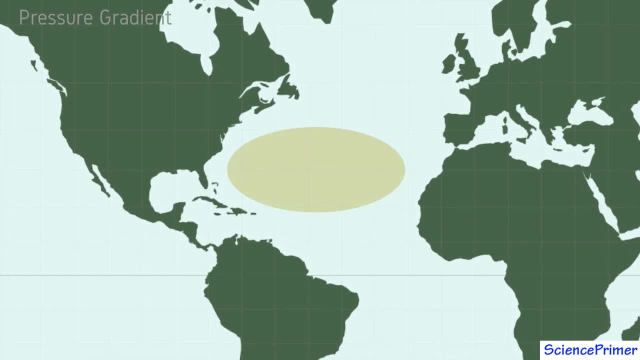 but this change in elevation is enough to generate a difference in pressure across the basin, with the elevated region in the center at a slightly higher pressure than the surrounding area. This creates a small pressure gradient across the basin. The pressure gradient acts like the hill.